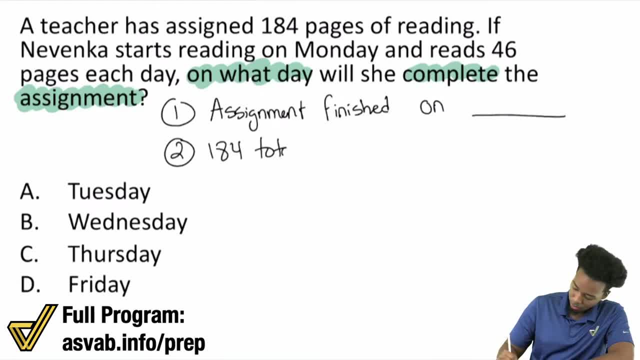 So we see here 184 total pages. That's right there Assigned 184 pages. My ASVAB party people. Hope you're enjoying the math party so far. Just wanted to remind you if you're interested in learning more about math. 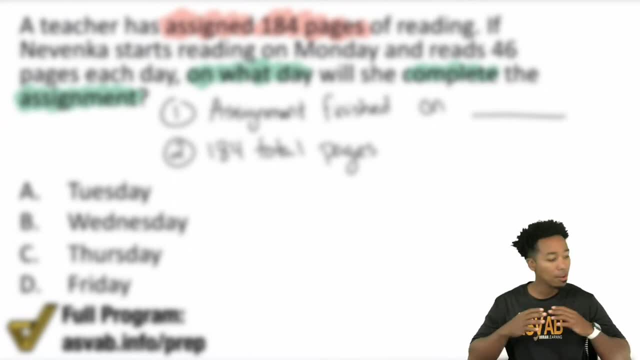 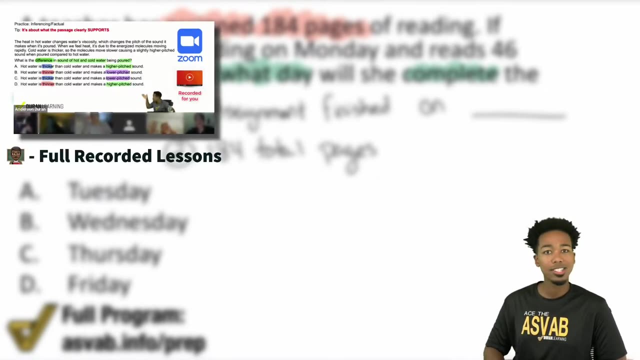 before we continue that, we do have a way for you to practice everything you need to get the ASVAB score that you want, Because in our math bootcamp we have everything you need in terms of recorded lessons to go through the entire concept. On top of that, we have guided practice. 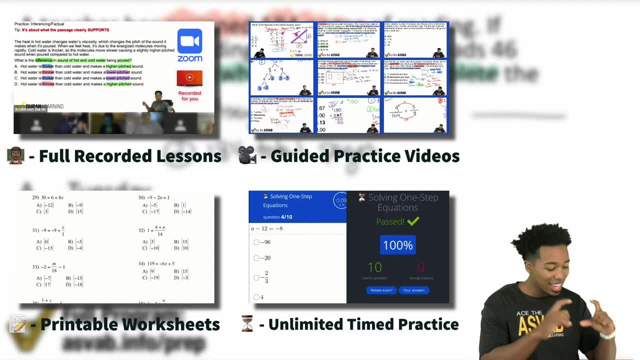 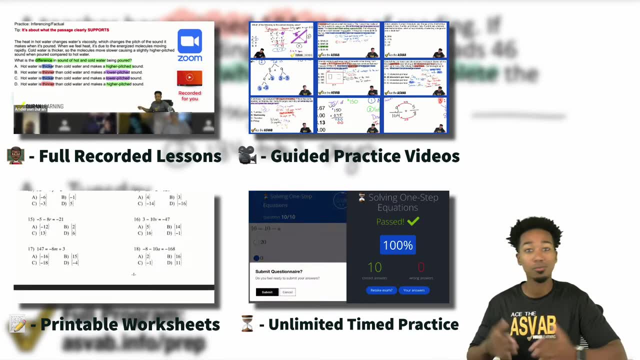 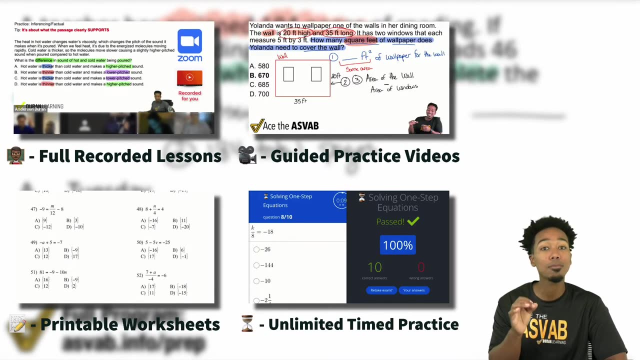 printable worksheets and speed drills for each and every single mini concept, from adding and subtracting decimals to fractions, distance rate, time, word problems, proportions, everything you need. It's all lined up for you learning as easy as possible, and we make updates to this course on a weekly basis at no extra cost. 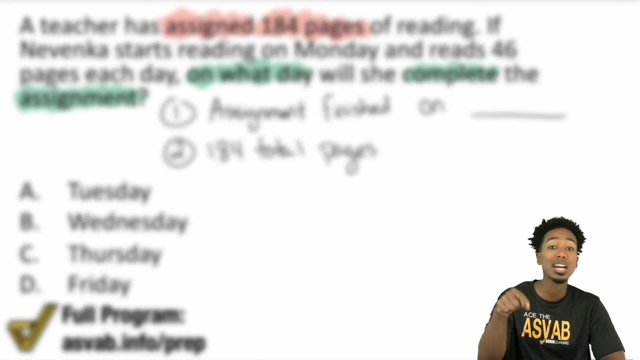 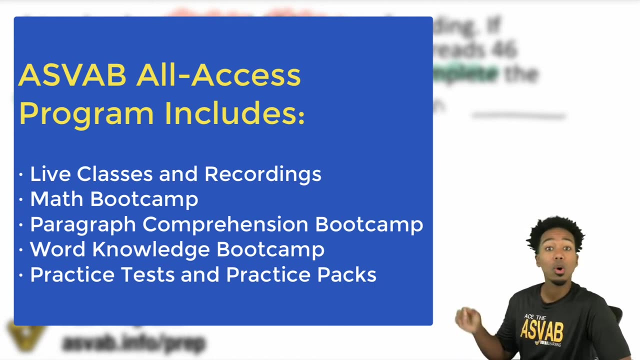 to you. So I really urge you and implore you, go ahead, check out the link in the description for the math bootcamp, which is also included in our full program, and we make it as affordable as possible. So go ahead, click the link in the description to learn about this more That way. 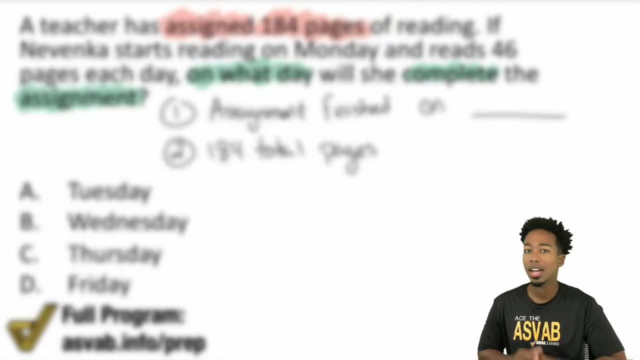 you know exactly what's available to you to raise your score. I don't want you to feel test anxiety. I don't want you to feel like you're lost and you're just hoping for the best. I want you to take control of your studying, and the ASVAB All Access program and the math bootcamp are the exact 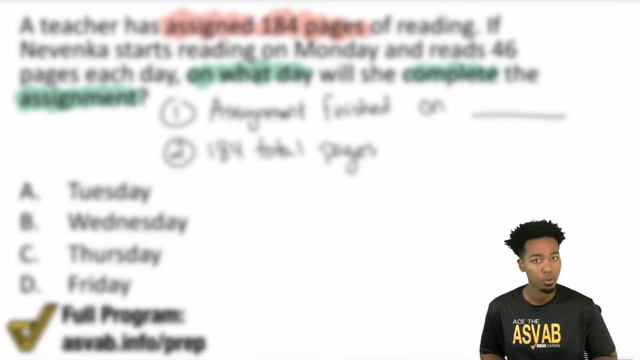 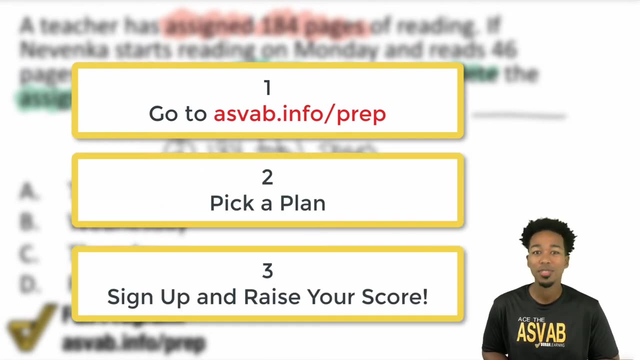 ways to do it. So if you have any questions, my contact info is also in the description, But before we continue, please check it out so you know exactly what's available to you. That way you can feel confident that there is a solution for you. Let's get back to the video, though. Let's 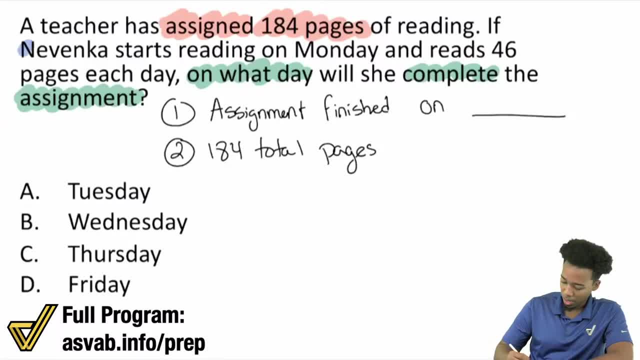 the ASVAB And then up next, we see that Nivanka starts on Monday and then reads 46 pages each day, or per day. Now, this is very useful information, because guess what Each day pages? each day, That's the same. 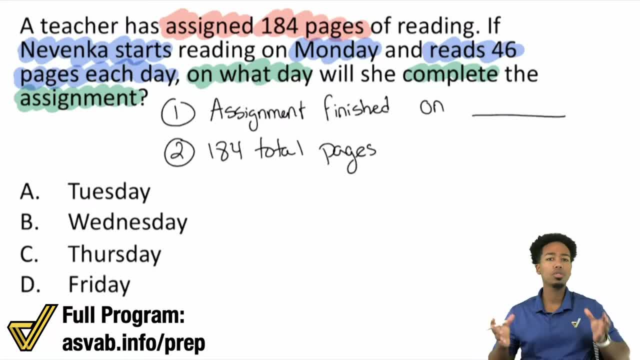 thing as saying pages per day. Now I'm going to review two different ways that we can solve this. The first way is going to be kind of like a caveman method, where you're kind of just using sticks and stones. Then the other method is going to be very useful in case we have a different. 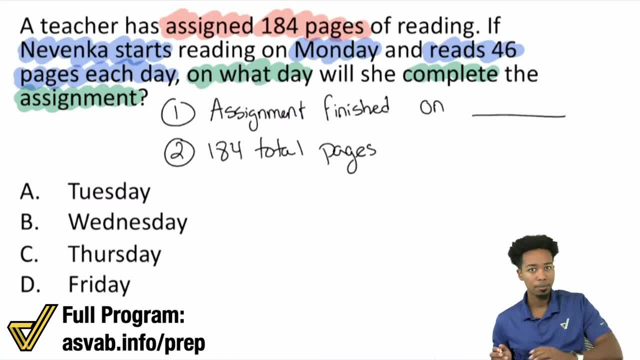 version of this problem, So let me show you the first way here. So, naturally speaking, I hope we can understand that. hey look, Nivanka starts on Monday, Right, Starts on Monday, And that's 46 pages each day. So on Monday we can assume that Nivanka 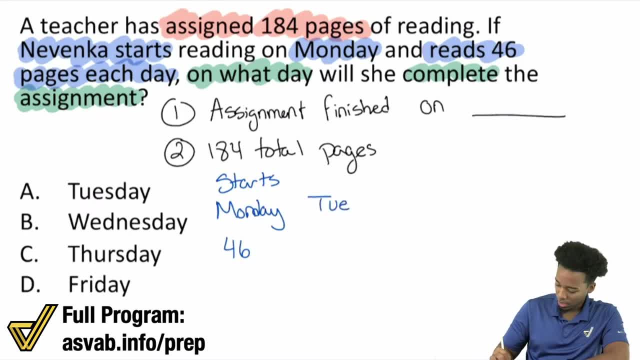 reads 46 pages. And then on Tuesday, that's another 46.. On Wednesday, that's another 46.. Thursday, another 46.. Friday, another 46.. And I'm not going to write anything more than Friday because you know, Friday is really the last day that we have as an option, So that's the last day that we 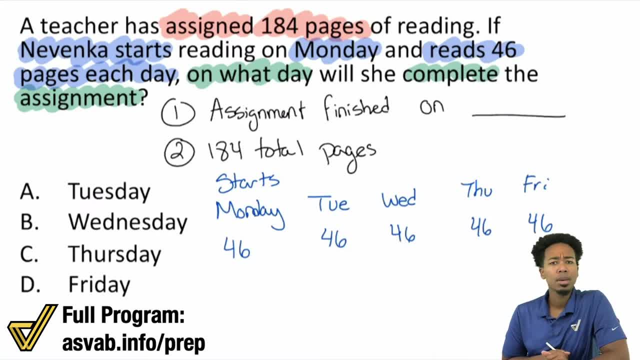 have as an option. No worries, we can stop right there. But here's the thing. This is the caveman method. I'm going to show you the faster method in a moment. But if you take a look here, you're saying hey, 46,, 46,, 46,, 46, and you're just going. 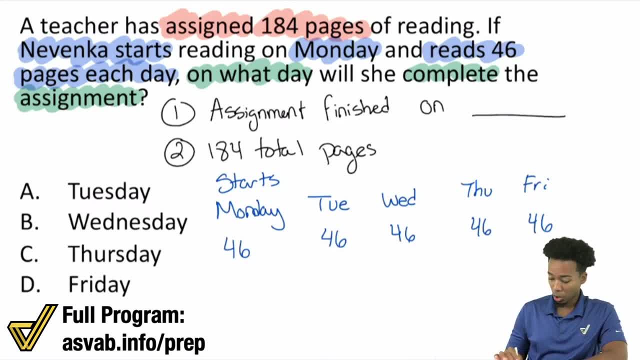 to keep adding up until you get to a total of 184.. That's it. So caveman method, here we go: 46 plus 46.. That's going to be what? Well, you can go ahead and do it on the side, if you'd like to. 46 plus 46. 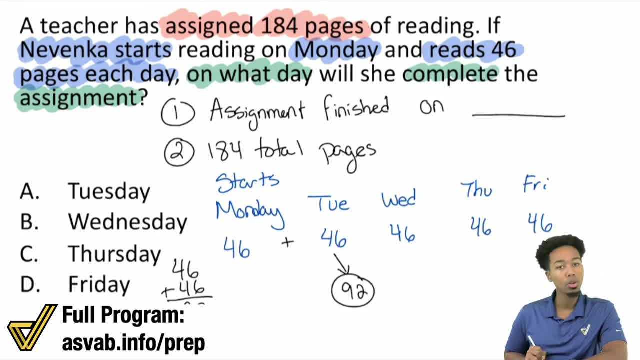 That's going to be 92. So we have 92 total on Tuesday. If you add another 46, what's that going to be here? Well, 92 plus 46. And you see how this is going to take a while right. 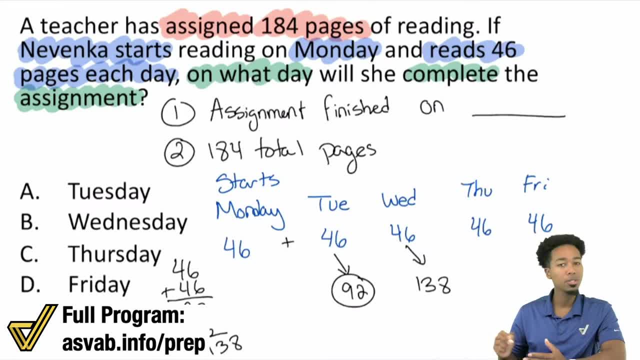 So that's going to be 138.. And again, you got to know your mental math a little bit, or you can go ahead and just do it by hand. Either way is fine. So then, if you have another 46, go ahead and add that now. 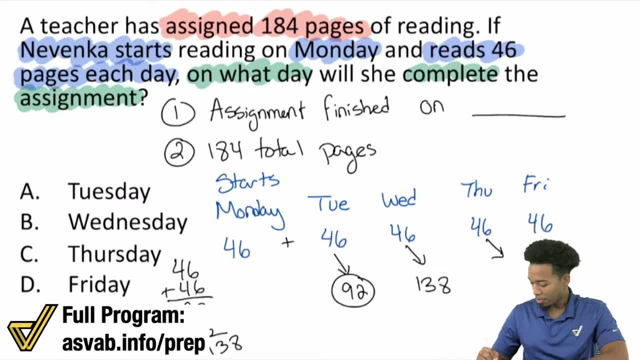 What's that going to give you? Well, that's going to be well, 40 plus 138. That's 178.. Then add the six, That's 184.. Oh, that's exactly what we need. There we are. 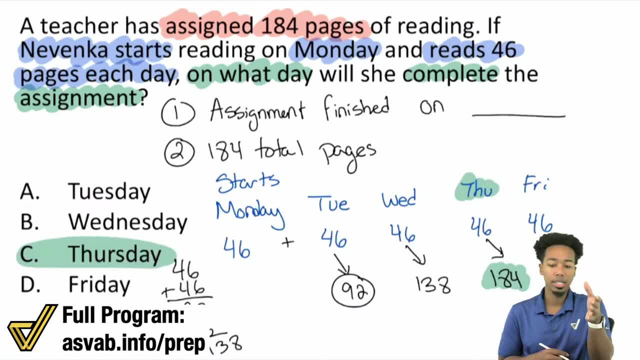 And that's going to be on Thursday. But here's the thing: I want to make sure that you know this clearly right now: What if? because when you're using the strategy obviously worked. but what if we're dealing with a problem that says, well, what if we have 2000 pages of reading, or 2,500, right? 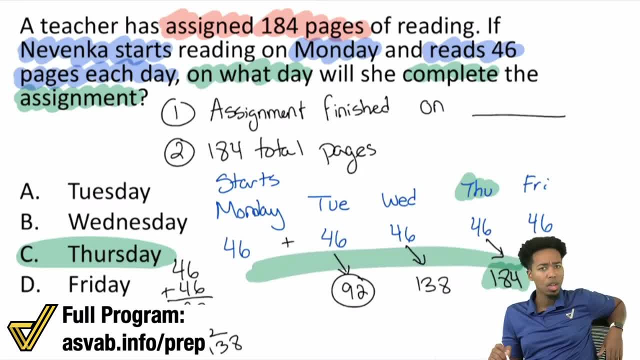 What if we have that many pages? Will this work? No, this is going to take way too long, And that's why I want you to understand that we should be able to see this as a distance rate and time word problem. So let me show you how we can set this up to get this done the proper way. 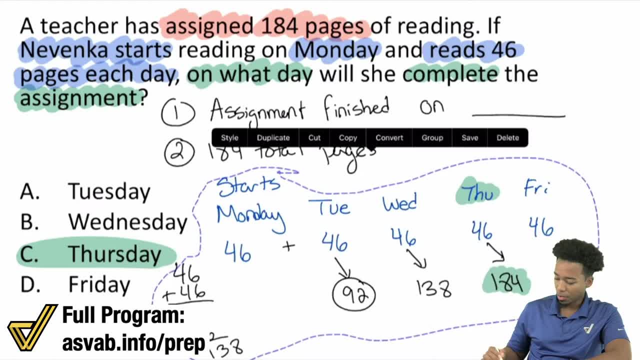 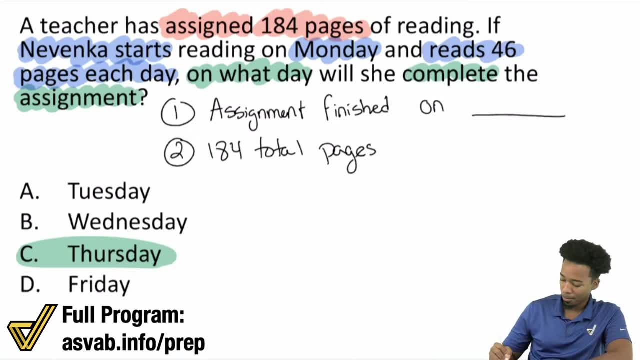 So here, here's what we can do. Allow me to go ahead and just erase everything that we've done. Feel free to rewind if you'd like to watch it again, But if you would like to think about it this way, I really implore you to do so. 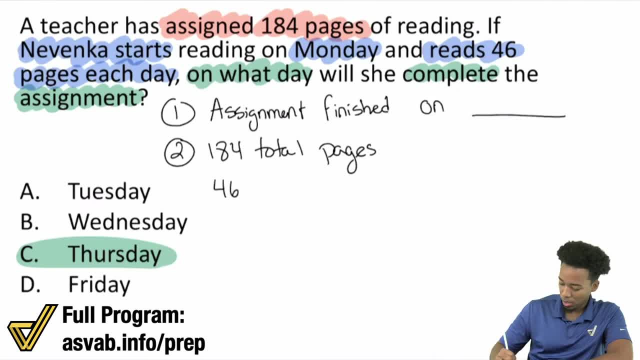 The 184 total pages. We have 46 pages each day, which is the same thing as saying per day same thing. And if you notice well, pages per day, we can consider that a rate. And then over here, 184 total pages, what we're trying to achieve, what the assignment. 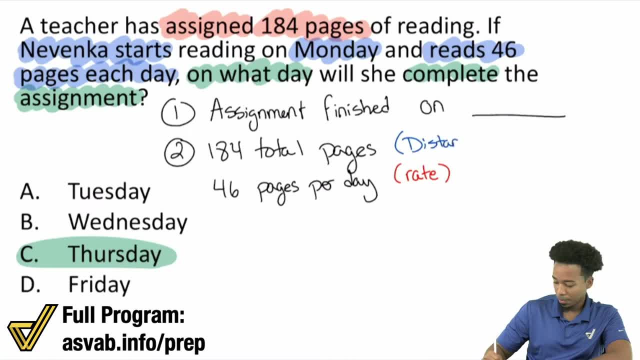 is the goal, that's considered a distance, And if you didn't know that, well, guess what? Again, whatever you're trying to accomplish is a distance: The speed at which you're doing it. That's the rate, And so what we're looking for is time, really. 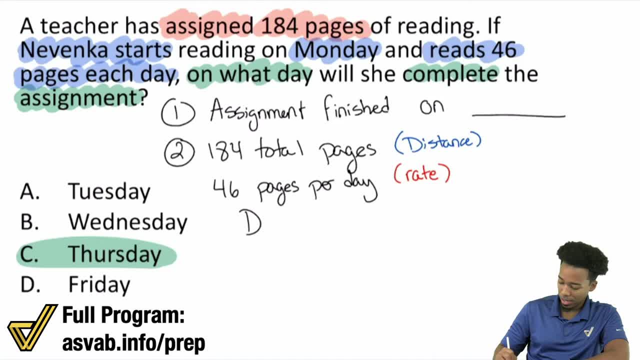 We're looking for time because if we set this up as a distance equals rate times time problem, guess what we can do? We have 184 equals 46 pages per day times the number of days or T for time. To solve this, all we need to do really is divide both sides by 46.. 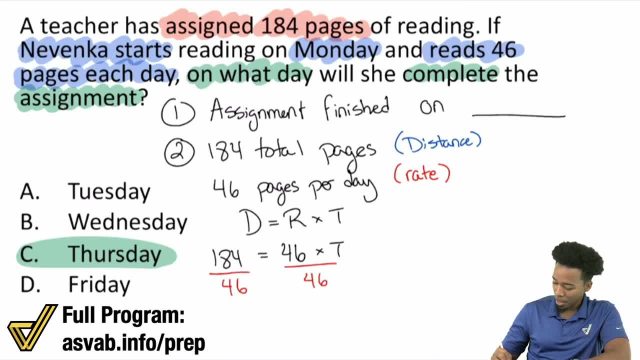 And guess what? We've got ourselves a nice good problem here, because we can cancel this out. We're going to do it on the right side, And then we just have to figure out what 184 divided by 46 is, And so to get that done, here's what we can do. 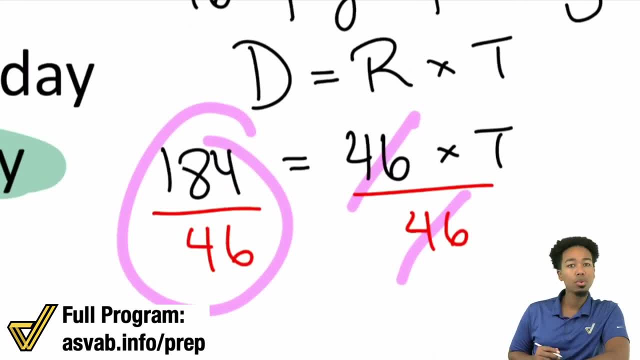 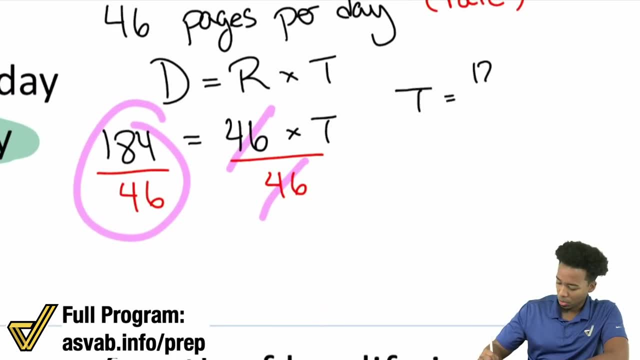 We can go ahead and say, hey, 184 and 46 are both even numbers. Since they're both even, we can actually simplify that nice and easy. And we can say: hey look, 184, 46, divide them both by 2 real quick. 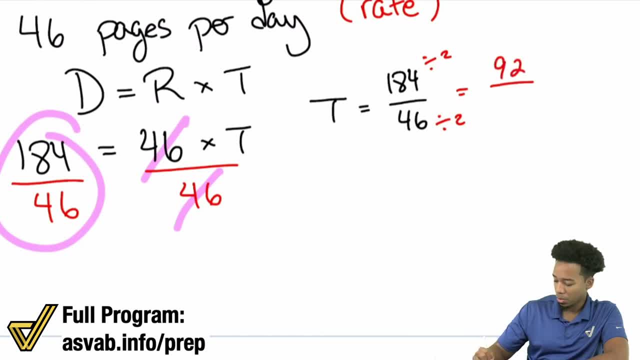 And if we do that, then we'll go ahead and receive Looks like that'd be 92 over 23.. All right, And then from there we'll see what we can do in terms of 23 going into 92. We can do a little bit of guesstimation if we want to.